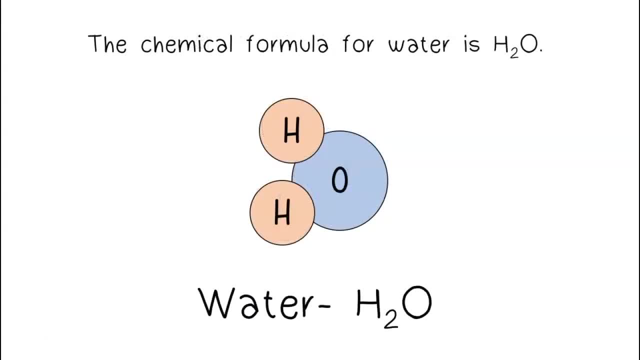 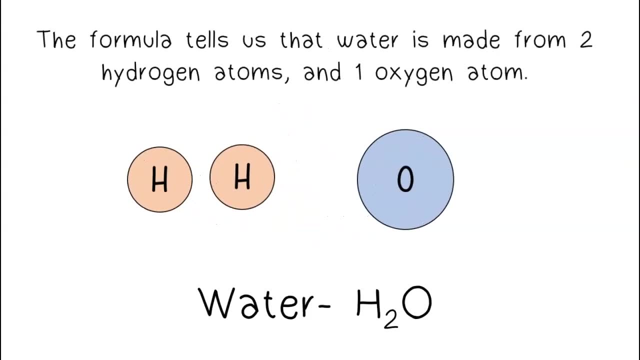 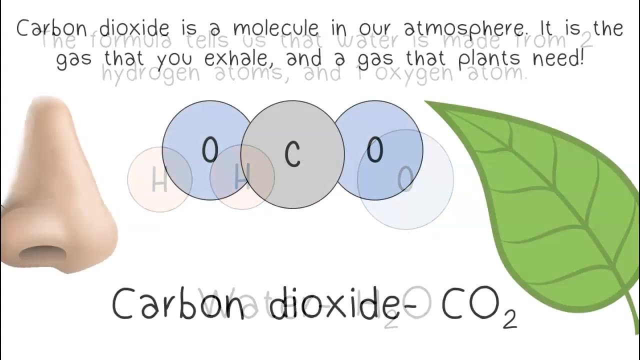 Water is essential for all life. The chemical formula for water is H2O. The formula tells us that water is made from two hydrogen atoms And one oxygen atom. Carbon dioxide is a molecule in our atmosphere. It is the gas that you exhale. 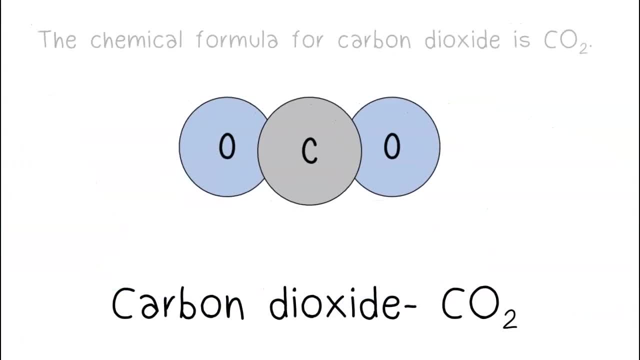 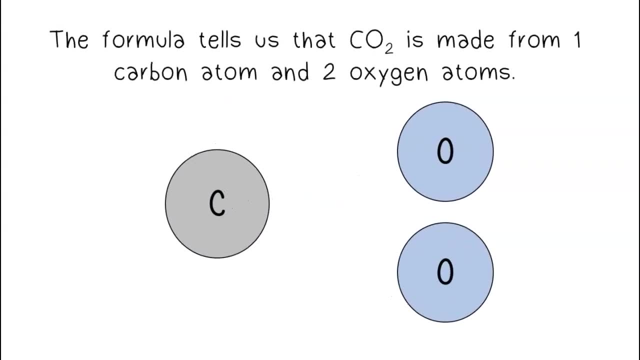 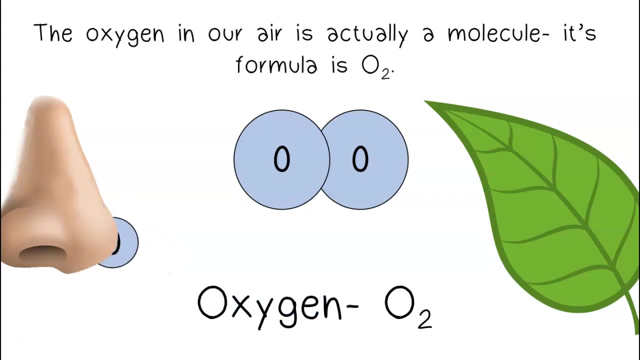 And a gas that plants need. The chemical formula for carbon dioxide is CO2.. The formula tells us that carbon dioxide is made from one carbon atom and two oxygen atoms. The oxygen in our air is actually a molecule. Its formula is O2.. 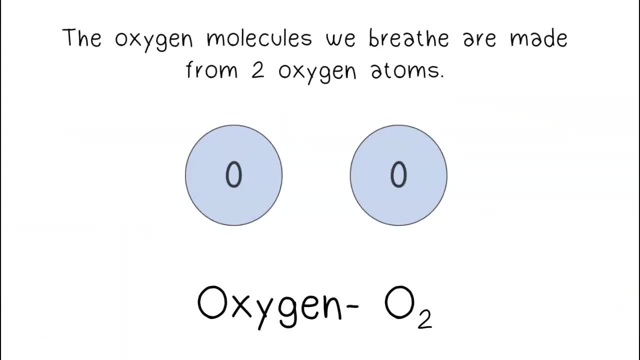 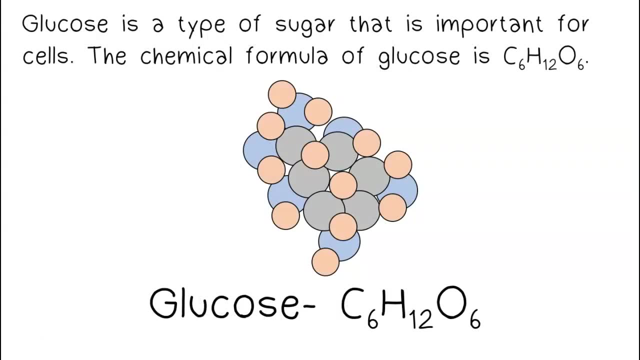 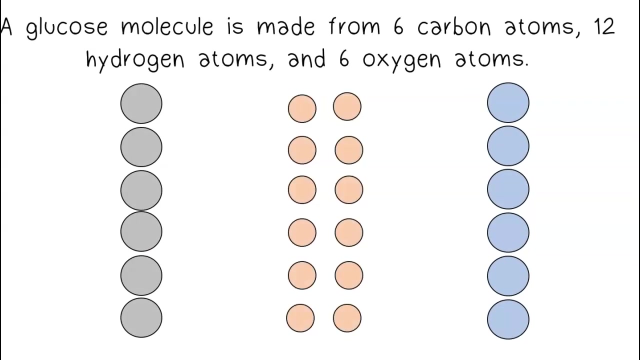 The oxygen molecules we breathe are made from two oxygen atoms. Glucose is a type of sugar that is important for cells. The chemical formula for glucose is C6H12O6.. A glucose molecule is made from 6 carbon atoms, 12 hydrogen atoms and 6 oxygen atoms. 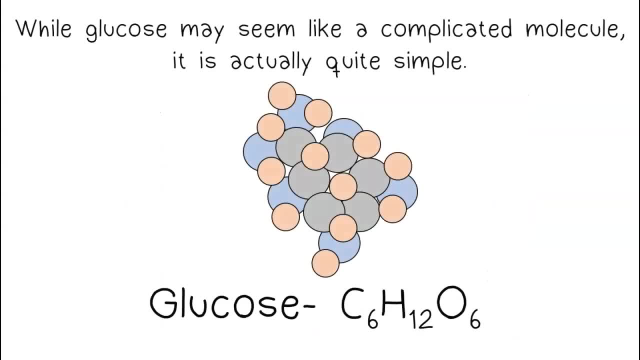 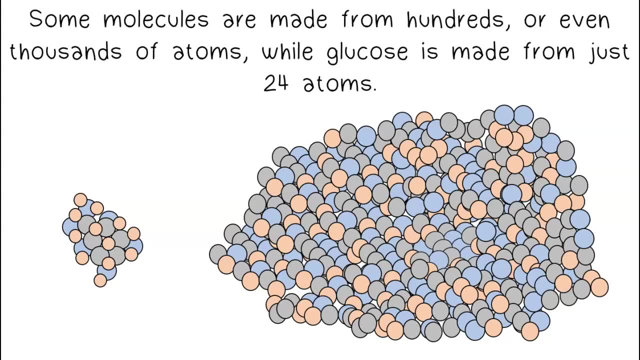 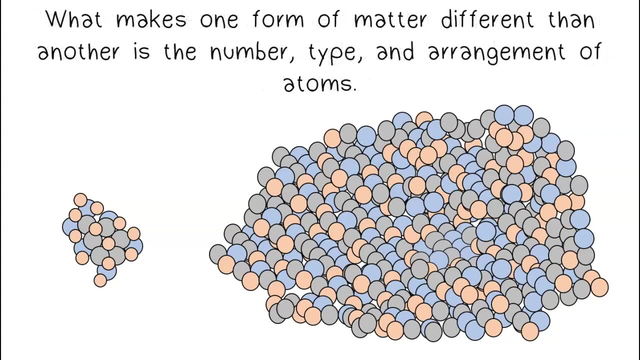 While glucose may seem like a complicated molecule, it's actually quite simple. Some molecules are made from hundreds or even thousands of atoms, while glucose is made from just 24 atoms. What makes one form of matter different from another? The number, type and arrangement of atoms. 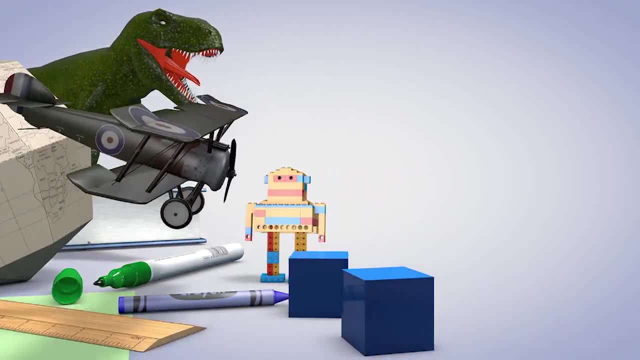 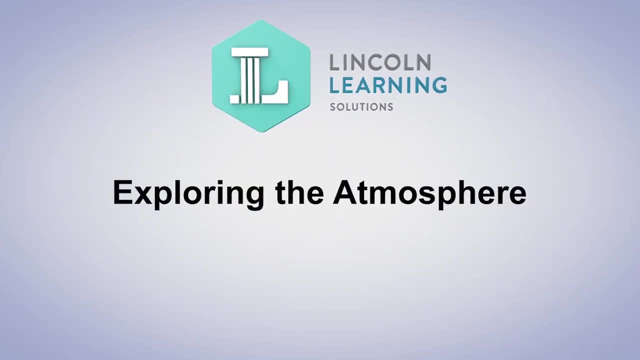 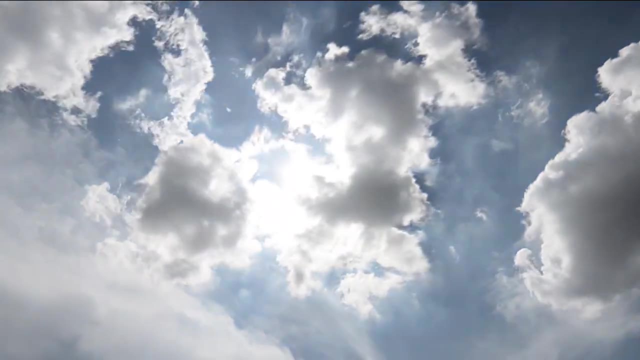 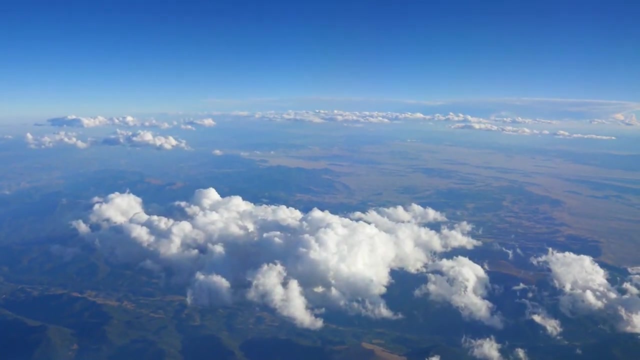 Whenever you look up in the sky, what do you see? At first glance, there might not seem to be much above you, Perhaps some clouds, the sun and a few birds. However, the most complex aspects of the sky above you cannot be seen. The very air itself that surrounds planet Earth is comprised. 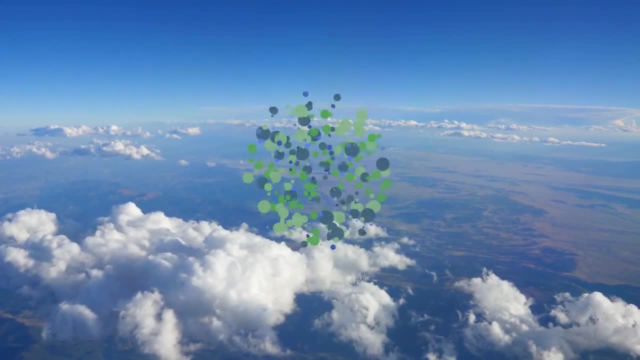 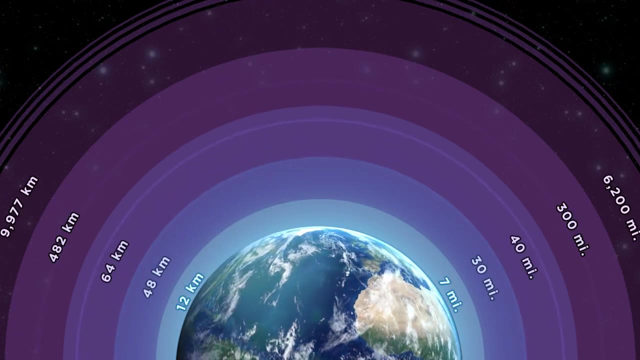 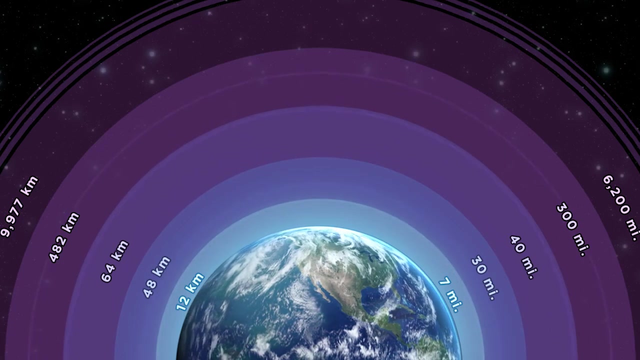 of a group of layers that combine to form the atmosphere. Earth's atmosphere is a blanket of gases that surround the planet. The atmosphere is made up of five layers. Each of these layers is unique because of the differences in temperature and particle composition. The